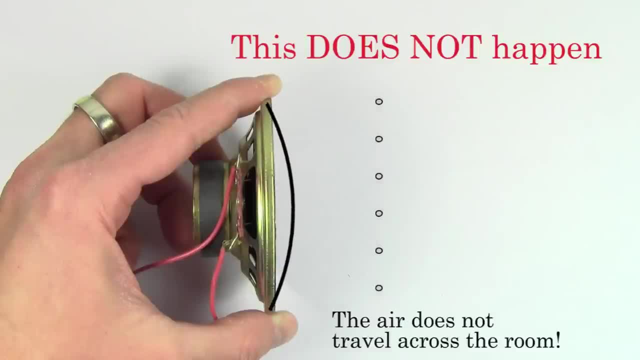 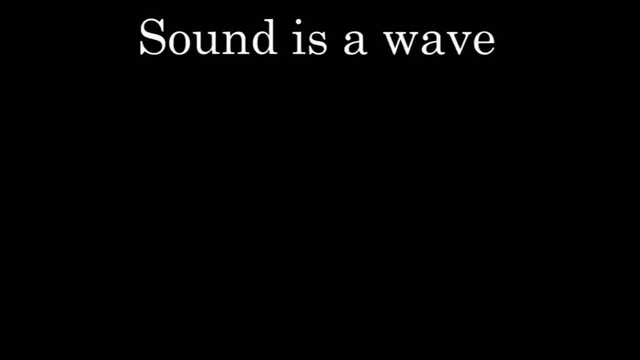 room here. but air itself is not traveling across the room, Only the disturbance within the air is traveling across the room. If air were being transported across the room, it'd be better characterized not as sound but as wind. So this is why we call sound a sound wave, because it shares the defining feature of 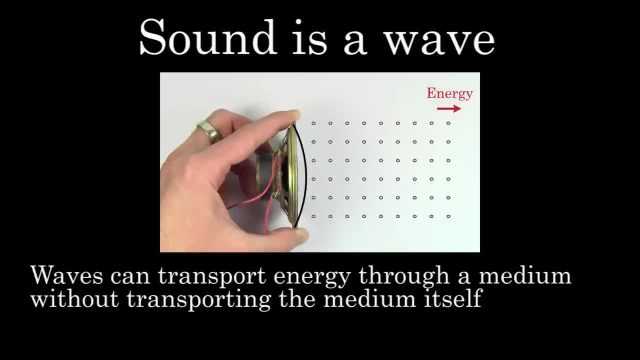 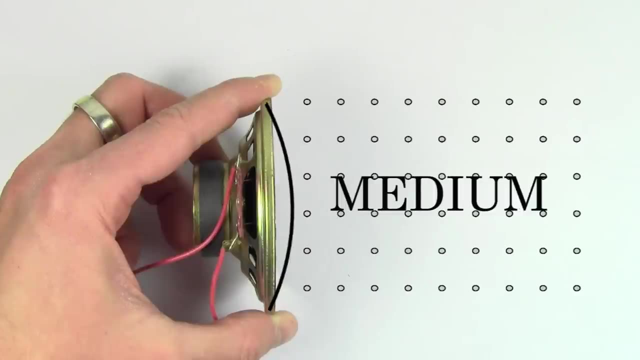 waves, Being able to transport energy through a medium without having to transport the medium itself. Medium is a fancy word for the material or substance through which a wave is traveling. Air is typically the medium for situations involving sound waves, but sound waves can travel through all kinds of different materials like water, metal or even human flesh, and 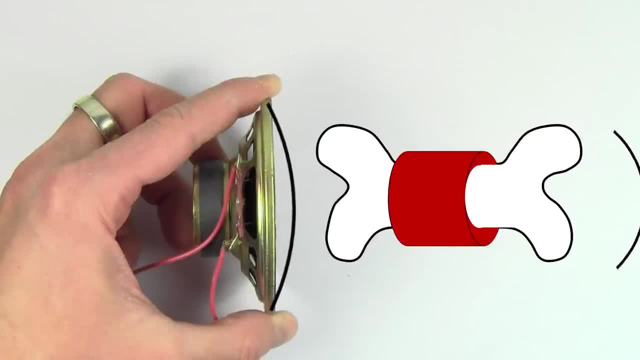 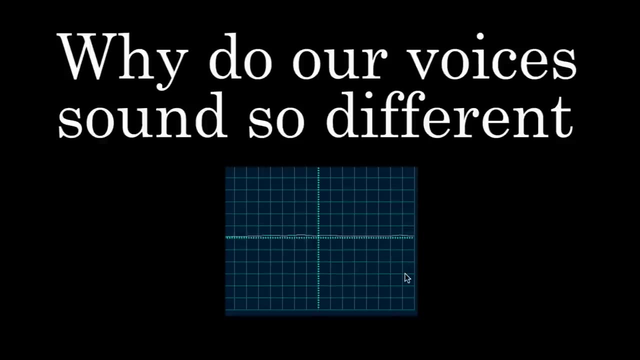 bone, And the fact that sound can travel through human flesh and bone explains something you might have always wondered about: Which is why do our voices sound so different on audio and video recordings? The reason for this is that when we're speaking to someone, we actually hear two contributions. 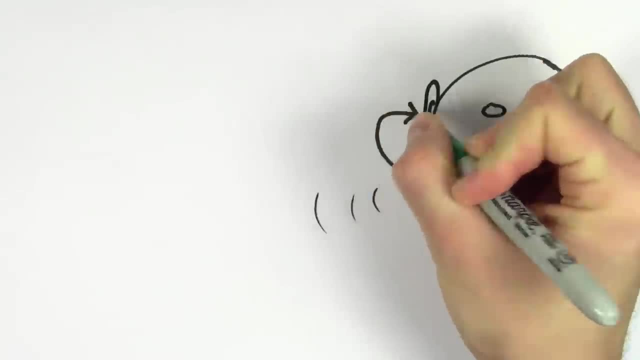 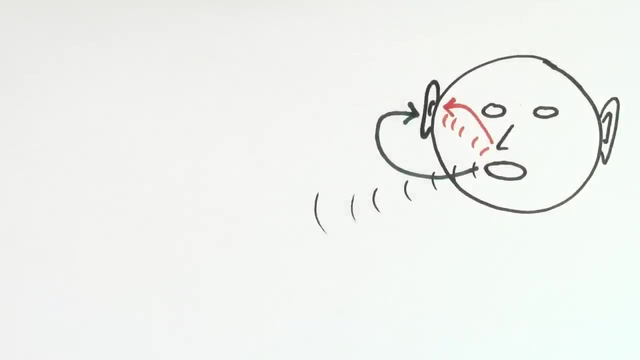 from our voice. We hear the sound wave traveling out of our mouth through the air and into our ear, But we also hear the vibration of the sound wave traveling through our flesh and bone, through our skull and into our eardrum. 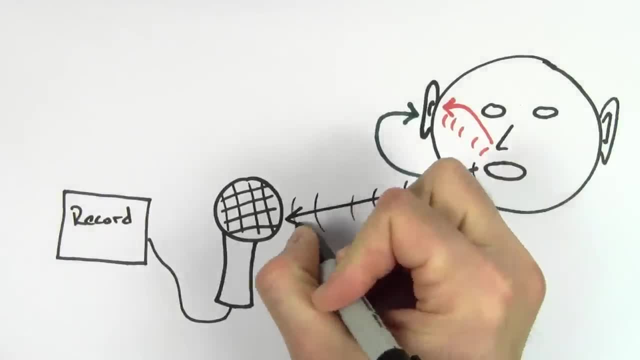 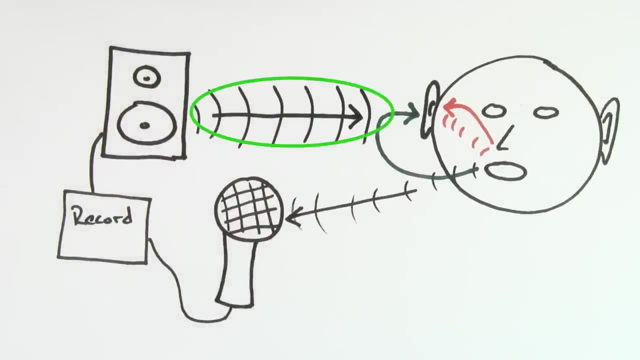 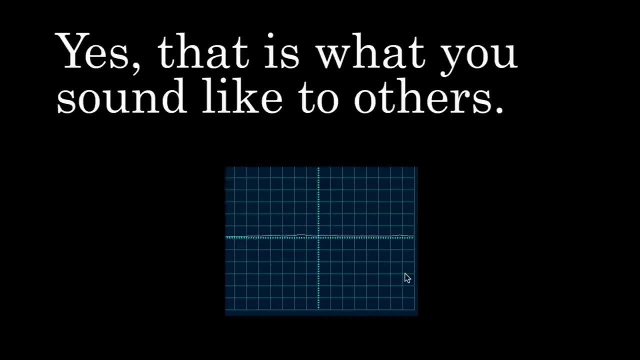 But on an audio or video recording, the only part that's recorded is the sound that travels through the air. So when you hear your voice played back on an audio recording, you only hear what other people hear when they listen to you. So the bad news is that, yes, what you hear on audio recordings is actually what you sound. 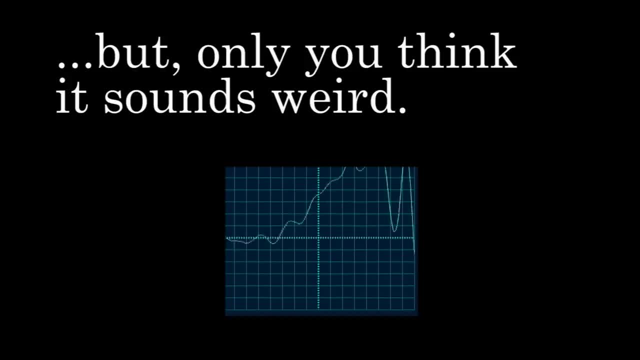 like to other people, But the good news is that most of your friends probably don't think it sounds weird, since that's the only voice they've ever heard you use, Unless you do actually have a weird voice, In which case I'll risk sounding pretentious by reminding you that you shouldn't waste. 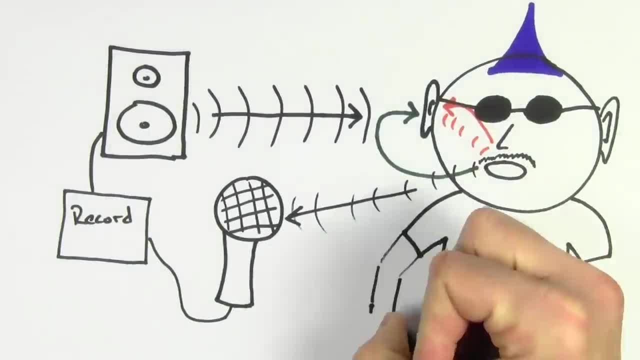 a lot of time worrying, Worrying about what other people think of you anyways.